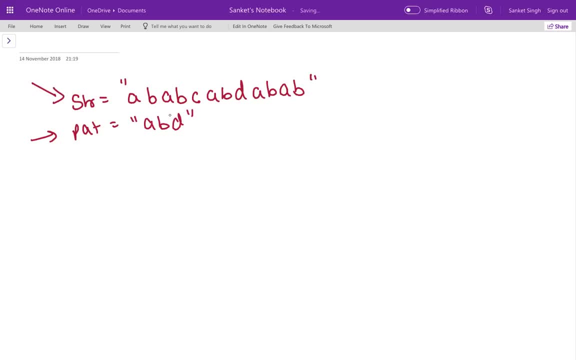 is present as a substring in this given particular string. So what our brute force approach says is that, for each possible position in this given string, for each possible position In this given string, What we are going to do is that we will check whether the pattern pat matches or not. 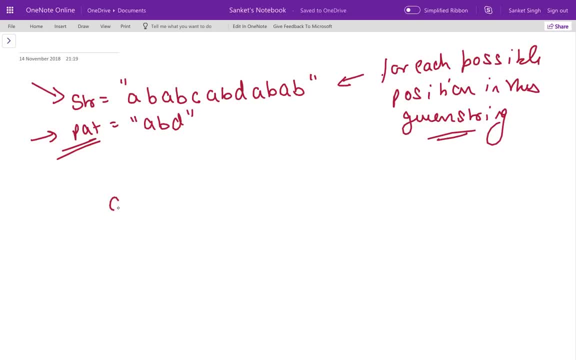 So what we are going to, what we are going to do is that in this given string, ab, abc, abd, ab, ab. Okay, So what we will do is that if the current character of the given string matches the first character of the pattern, then we will try to iterate over the whole pattern and 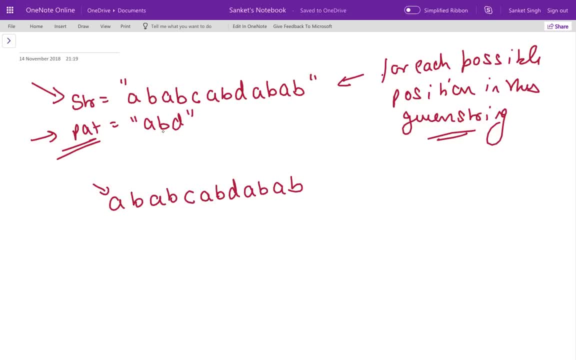 the whole corresponding string and check if there are any inequalities in the characters of the pattern and the string or not. And if we are not able to find any inequality, then we can return true that this pattern is present as a substring in this given string. 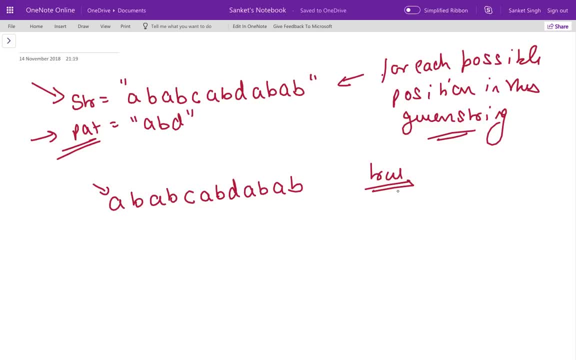 Okay, So what we are going to do is that we will try to iterate over the whole pattern and the given string, or, if we are able to find any inequality, then what we will do is then move on to the next corresponding character and then repeat the same process. 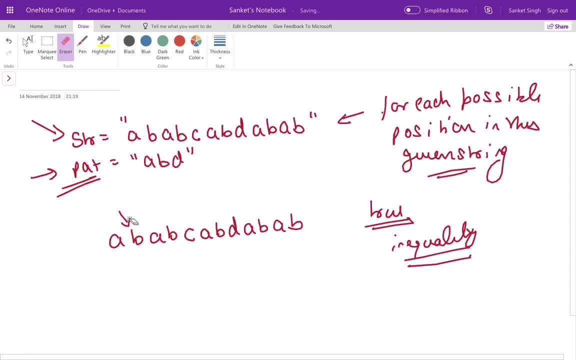 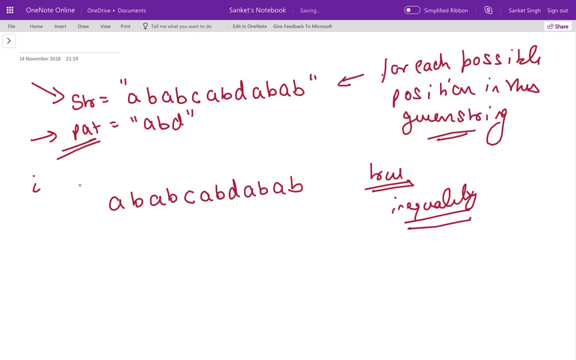 So let us iterate over this short example and see how the brute force is working. So the first character of. let us take a pointer i, and now i is pointing to the first character of the given string. so if the first character of the given string matches the first character, 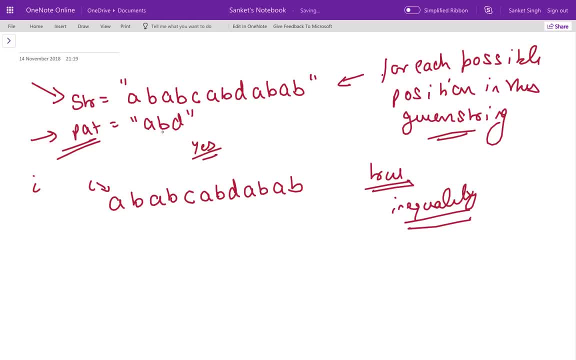 of the pattern- yes, it matches. then what we will do is check if the second character of the given pattern matches the second character of the string. yes, it matches. then the third character of the pattern matches the third character of the string or not? and no, here we found an inequality. 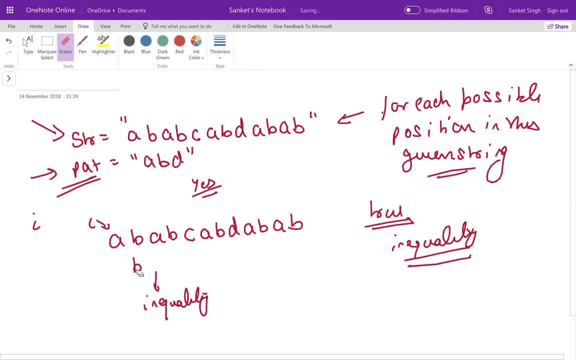 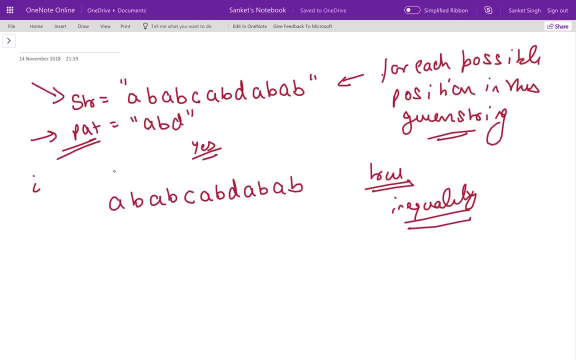 So what we will do is increase our pointer i that was initially pointing to a and now i will be pointing to b. and now here we will check that if the ith character of the given string matches the first character or the pattern or not, and hence here we cannot find any match, so we will increase our i. 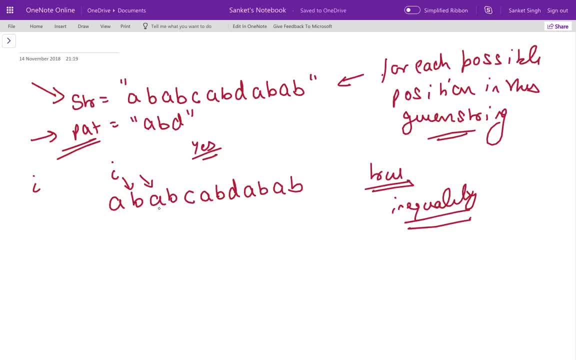 again, and now i is pointing to the third character of the given string. now, if the ith character of the given string matches the first character of the pattern- yes, it matches. then we will check if the i plus 1th character matches with the second character or not. and yes, it matches. and 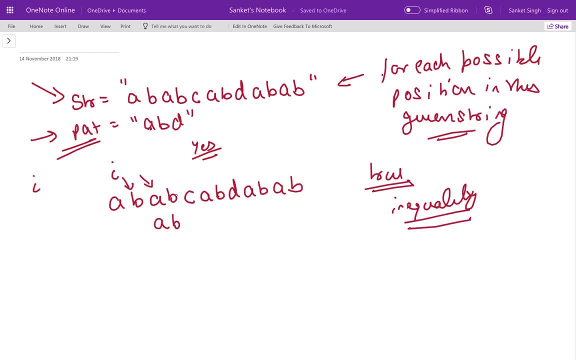 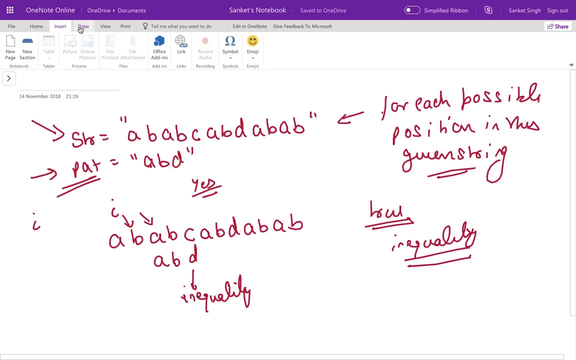 then we will check if the i plus third, i plus second character, that is this c, matches with the third character of the pattern, that is d. so here we will again found an in. so now, what we will do is then again update our i, that was pointing to a, to now point to this b. 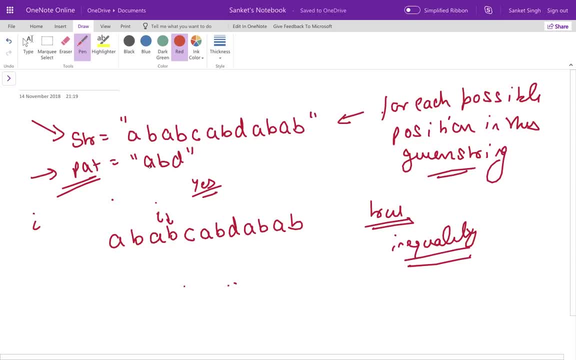 so we will check if the ith character matches the first character of the pattern or not, and hence it does not matches. so we will again update i. so we will check if the ith character matches the first character of the pattern or not, and here also it does not match. so what we will do is again update i. so now i is pointing to this a, so we 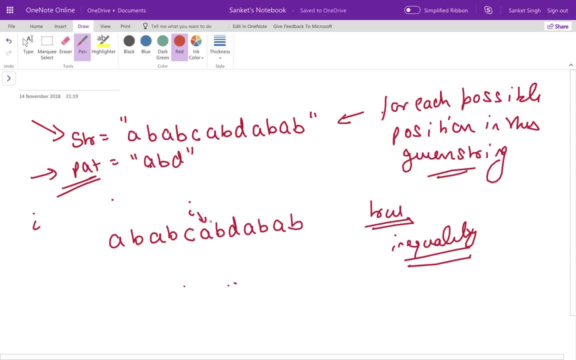 will check if the ith character matches the first character of the pattern or not. and yes, it matches if the i plus 1th character, that is this b, matches with the second character of the pattern, that is b also. so yes, it matches. and now we will check if the i plus 2th character, that is this d, matches. 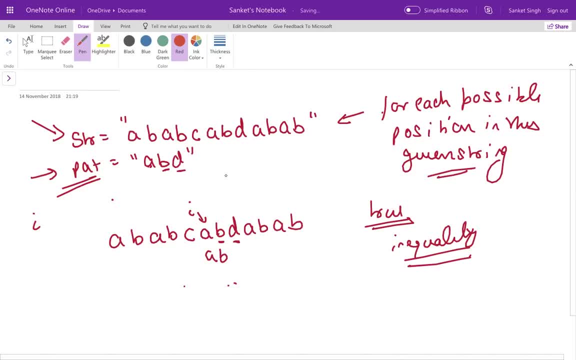 with this particular third character of the pattern or not. and yes, it again matches and you can see we are at the last character of the pattern. so we have found an index where the pattern is present as a substring in the given string. so we will return i as the index at which we have found. 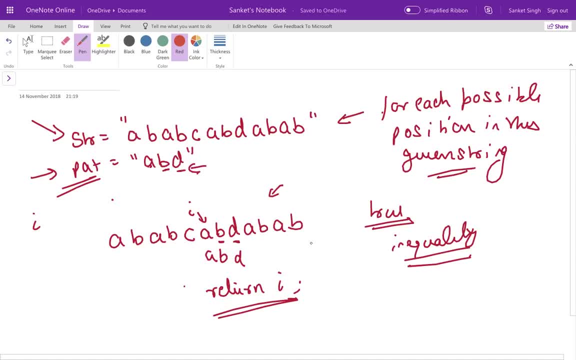 this pattern. so here you can see. in the worst case what we are going to do is for every character in this given string, we will check if the pattern is present or not. so in the worst case what we will be doing is we will be iterating over n minus m elements. suppose n is the length of string and 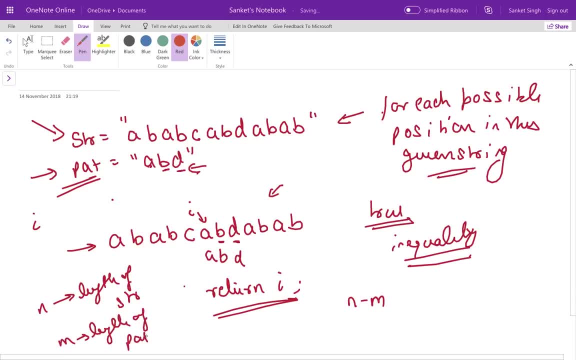 m is the length of pattern. so we will be iterating over n minus m elements of the given string, and for each character in this element we will be iterating over m characters, at most m characters of the given pattern. so the time complexity here will be big. o of n minus m, which will be 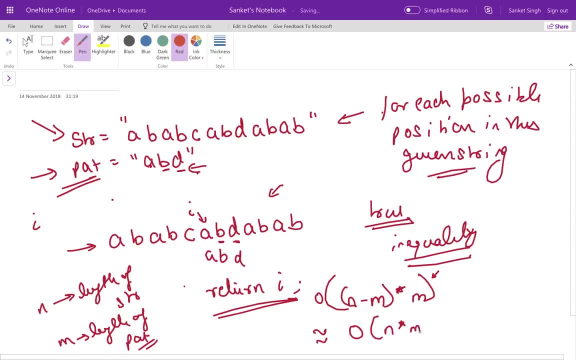 near equal to big o of n into m, and suppose for cases where m will be nearly equal to n, this complexity will shoot and becomes big o of n square. so the brute force approach for pattern matching is giving us big o of n into m time complexity. 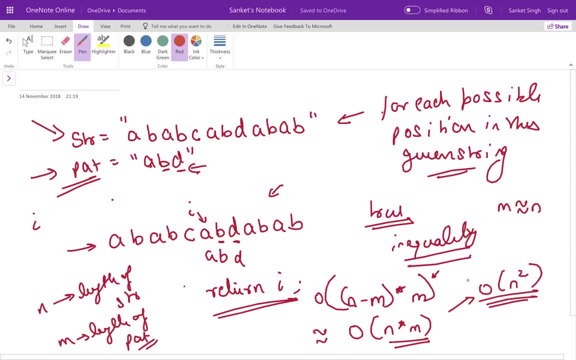 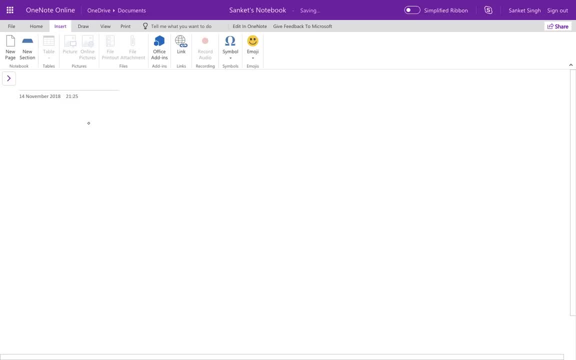 and for m nearly equal to n, this will give us big o of n square. so can we improve this? yes, we can. so here comes the Rabin-Karp algorithm into the picture. Rabin-Karp algorithm. so let us first know about a very interesting concept that is rolling hash. 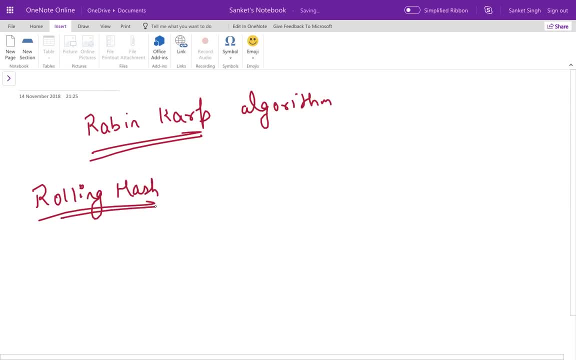 so Rabin-Karp algorithm is based on rolling hash technique. so what rolling hash says is that suppose we have a hash function which takes an input, a string, and gives a unique hash, let us say x, for that particular string. so suppose we are given a string like a, b, a b, c, a, b, d, a b. okay, so suppose 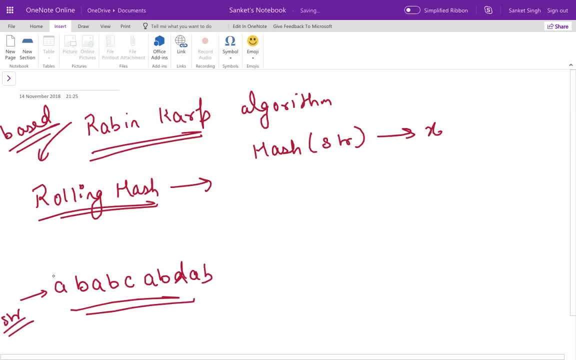 we are given a string like this and let us mark the indexes as 0, 1, 2, 3, 4, 5, 6, 7, 8 and 9. so suppose for a substring of this given string, starting from character 1 and ending at: 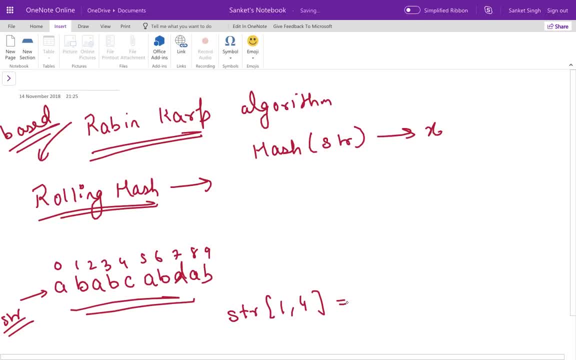 character 4, where 1 and 4 are included. so this substring will be b a, b, c. suppose we calculate the hash value of b a, b, c and this hash value comes out to be, suppose, any integer or long value, y. so if we know the hash value of a given string, of a given substring, starting from index i and 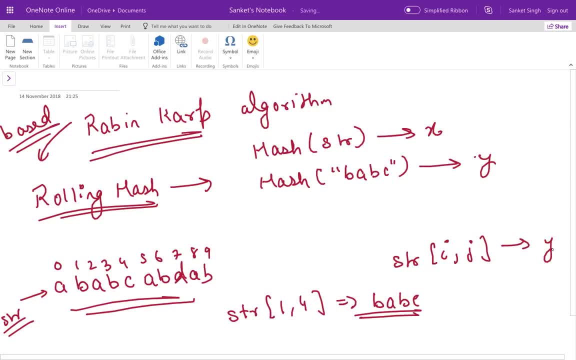 ending at index j and let us say the hash value is y. so if we want to calculate, calculate the hash value of a given substring, starting from index i and ending at index j. calculate a new hash for the string, starting from the i plus 1th character to the j plus 1th. 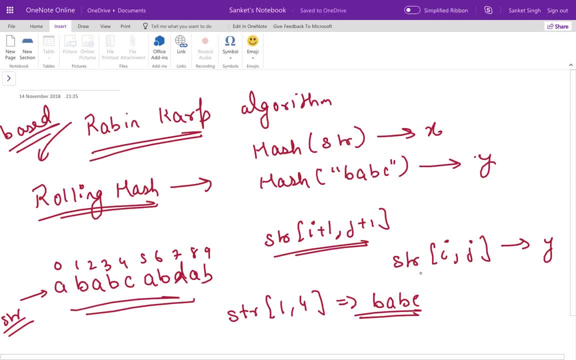 character. so what we are supposed to do is that we know the hash value of the substring starting from index i and ending at index j, and now we want to calculate the hash value of the i plus 1th index, the substring starting from the i plus 1th index, to the substring ending at the j plus. 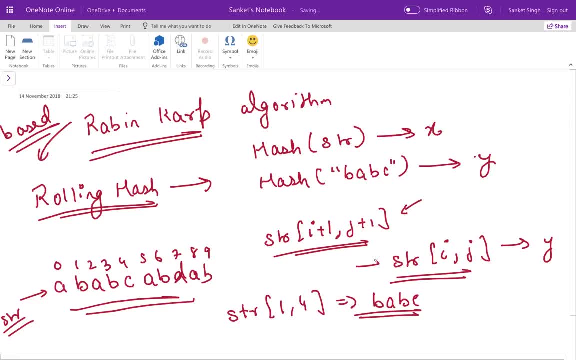 so what the rolling has says: by already knowing this particular hash y, we can calculate the hash of this substring starting from i plus 1 and ending at j plus one in O of 1 time complexity. so how can we achieve this? let us see a very quick example. suppose for the substring 0 to 2, that is, a, b, a. let us define a hash function under the: Because i is equal to, i equals i plus number and the hash of the j plus 1 weiter becomes j plus number over the –yché value of j plus 1 in the non- delta. 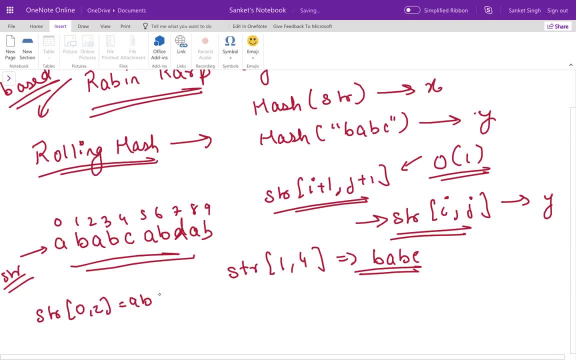 0 to 2, that is, ABA. let us define a hash function which only does a simple thing, that is, adds the ASCII of the characters. okay, so what we are doing here is just adding the ASCII of each character of a given, of a given substring, for which we 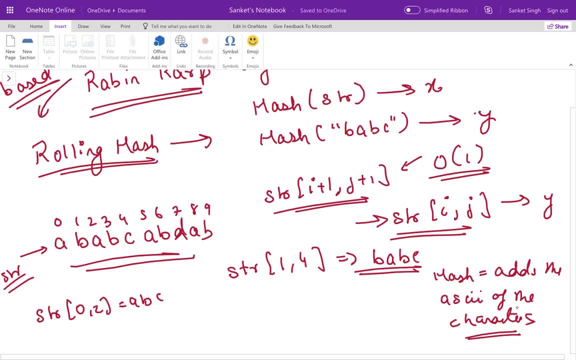 have to find the hash value. so here three characters are ABC. so when we will pass, pass these characters ABC in our hash function, what it will be it will be doing is that it will add all the ASCII's, that is, ASCII of A, B, A and C together, and it will be giving us a unique hash value. so let us say we are. 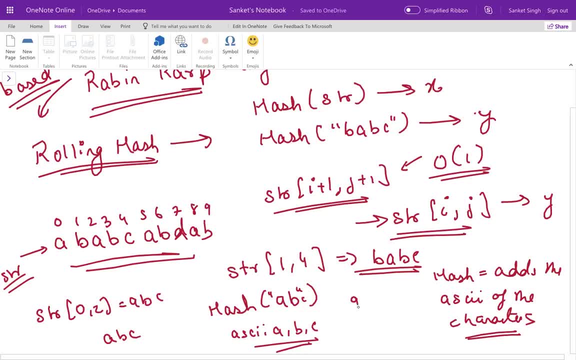 adding the ASCII of A, B and C. so ASCII of A is 97, B is 98 and C is 99. so by adding the ASCII of A, B and C, that is, 97, 98 and 99, we will be getting the hash value as 294. okay, so here we can easily see. 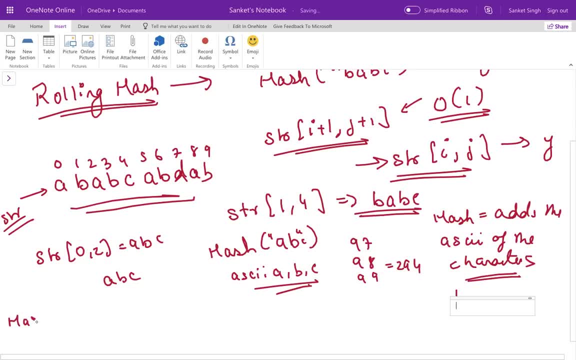 that the hash function gives the ASCII of ABC as 294. so now if we want to calculate the hash value of the substring starting from 1 and ending at 3, that is BAB, and we already know the hash value of ABC. so what the rolling hash function will do is that calculate this as this hash value of BAB. 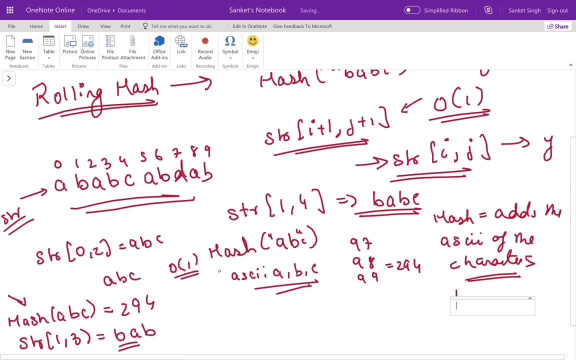 in big of one how it will do that it is. it is simply seen that if we subtract the ASCII of the first character of the original string, that is, the hash value was 20: 294, and if we subtract the ASCII of a and add the ASCII of B, then we will. 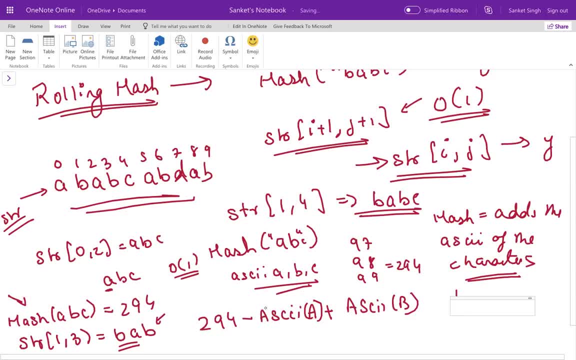 be easily find able to find out the hash value for BAB. so 294 minus 97 plus 98. so by subtracting 97 and then adding 98 we will be able to get a unique value that is 295. so here you can see, we are easily able to get the hash value for the next. 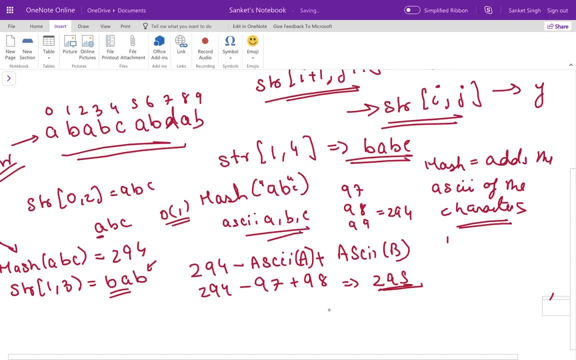 string in big of one time complexity. so let us take another example for the next corresponding string in big of one time complexity. so here you can see we are substring, that is, substring starting from 2 and ending at 4. here now we already know the hash value for BAB and substring starting from 2 and ending at. 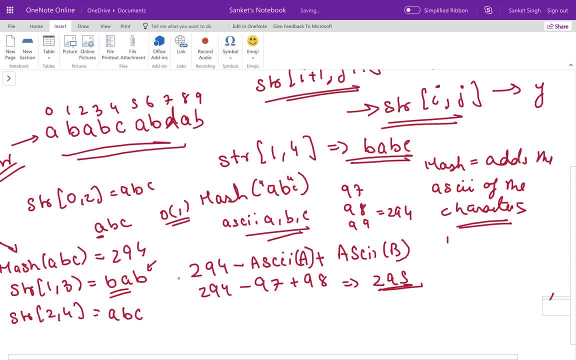 4 is ABC. so what we will do is subtract the ASCII of the first character of the previous string, that is ASCII of B will be subtracted, and now we will add the sub ASCII of the last character of the new string, that is ASCII of C will be. 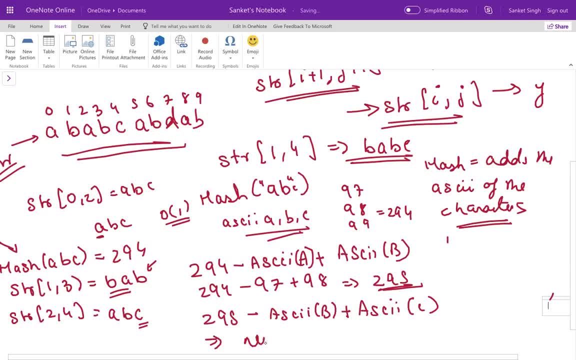 added. so here you can easily get the new hash value. so here you can see the rolling hash function is very, very efficient in calculating the new hash values if it already knows the hash value of the previous substring. so our Rabin-Karp algorithm is completely based on this rolling hash. 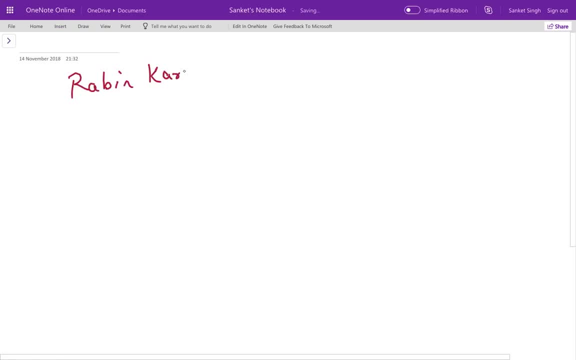 technique. the Rabin-Karp algorithm is based on the rolling hash technique. I hope you already- you all- have got a clear idea of what rolling hash technique is, and now we will look at the Rabin-Karp algorithm. so what Rabin-Karp algorithm will? 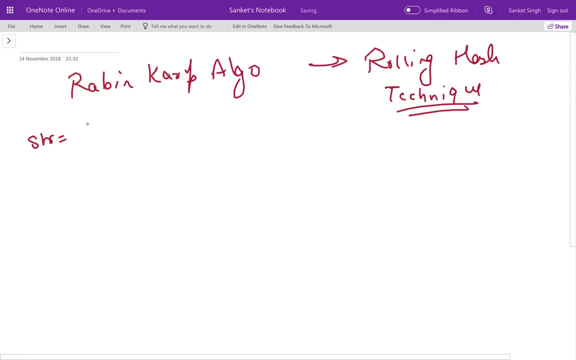 say is that suppose we are given a string as ABC, ABD, AV and we have been given a pattern that is ABD. so suppose we will write our unique rolling hash function and we will not be using the addition of ASCII function. we will write something else. so suppose we will write a hash function that will take 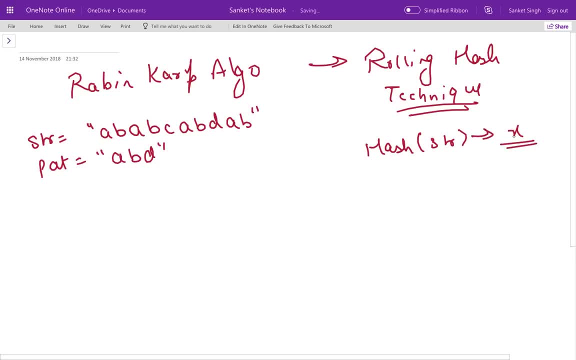 take a string and splits out a unique hash. so in Rabin Karp algorithm, what we will do is that first calculate the hash of pattern, so we will calculate the hash of given pattern. then in the next step, what we will do is calculate the hash of. 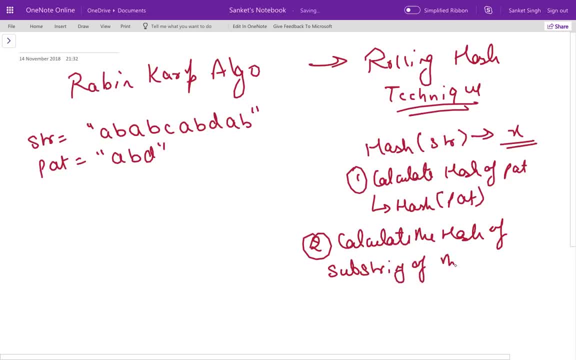 substring of the given string, starting from index 0 and ending at index pattern dot length minus 1. so what I am trying to say is that initially we will calculate the hash of this given pattern and we will then calculate the hash of the substring starting from the 0th. 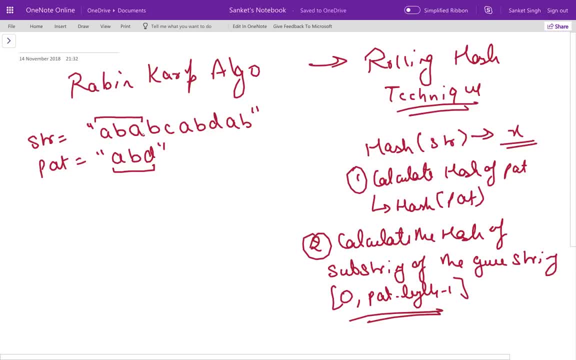 character and ending at the pattern minus 1, 1th character. so here the length of the pattern is 3 and pattern dot length minus 1 will be 2. so we will be taking the substring 0 to 2 and we will calculate the hash of these two values. so these two steps will take big O of m time as the length 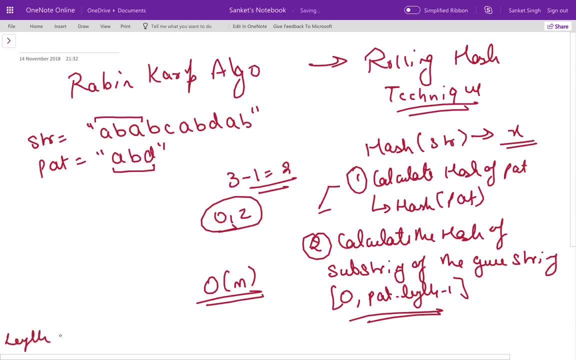 of the pattern. suppose length of pattern is m, then calculating the hash. we will not be using the. calculating the hash for this pattern will take big O of m time as initially all we have to calculate the hash by iterating over the whole pattern and then again the using the substring of. 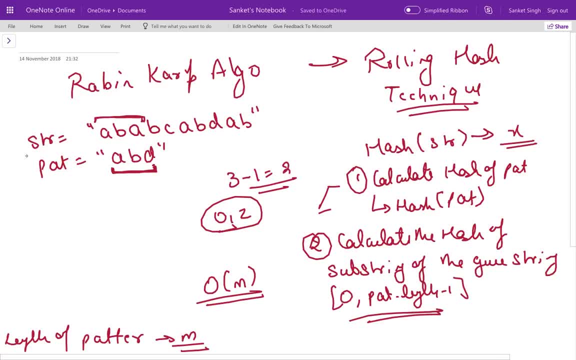 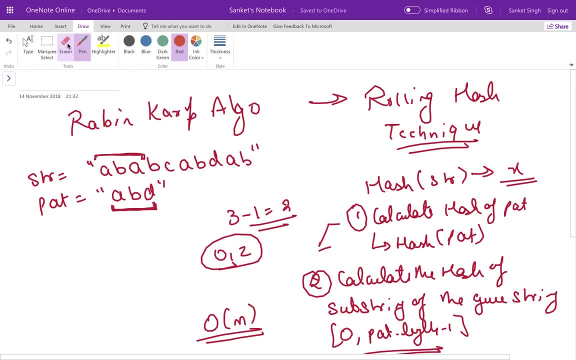 length m from this particular given string, we will again calculate the hash of the substring. so these steps will take big O of m time. and now what Rabin, repeating multiple times, will take big O of m times. and now what stabicarp says, is that at each step, after calculating the initial hashes, what we are going to do, 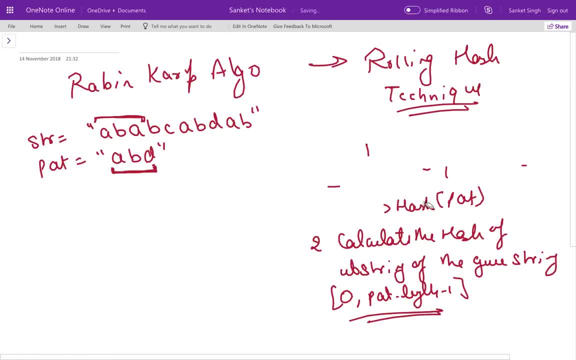 let me pick up all the steps. so what our Rabin calculating Thom defender algorithm says? that at each step, since we are finding the hash of M characters, that is, the length of the pattern in the given string, we are using an rolling hash technique to calculate the given hash for the given string. so what we 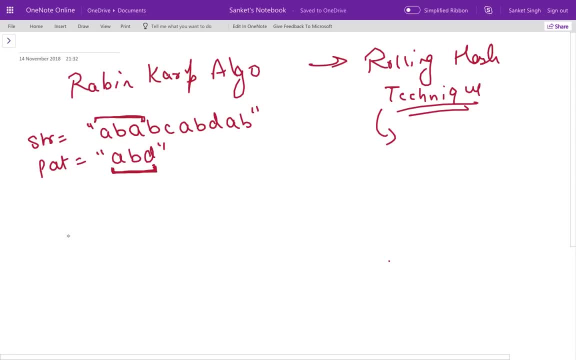 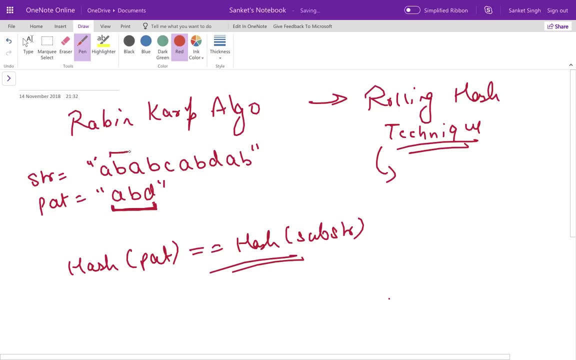 will do is that at each step we will check if the hash of the pattern matches the hash of the substring or not. if the matter is not found, then we will iterate this particular window to the next eligible substring. so again we will calculate the hash of this substring. and here you can see initially: 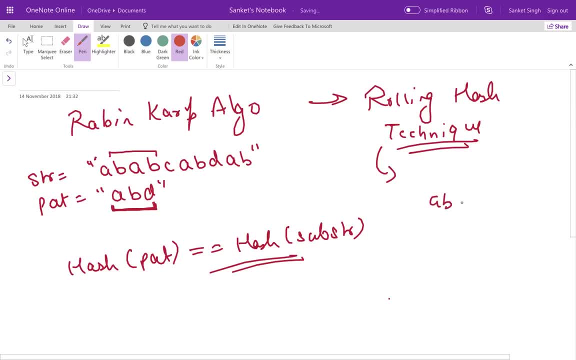 if we had the hash value for a ba- and now we want to calculate the hashtag value for a- and again, you can see we have these two hash values and we can for BAB- then this will be done in O, So we will calculate the hash of the next. 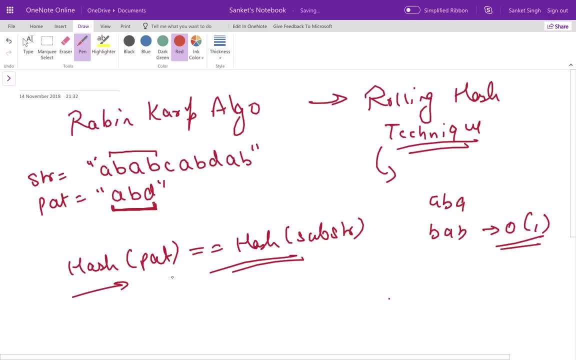 eligible substring and we will check if the hash value of the pattern and the hash value of this new substring matches or not. Suppose it does not matches, then again what we will do is shift the window to the next eligible substring and if at any point, if at any particular 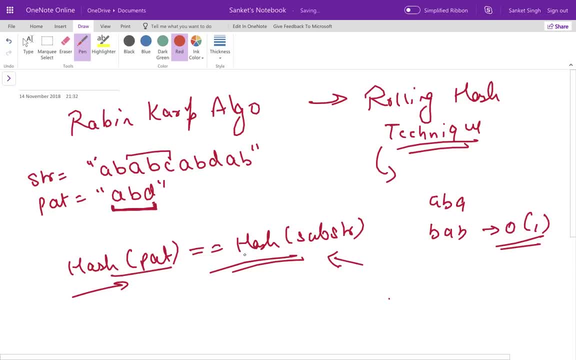 point, we found that the hash value of the pattern matches the hash value of the substring. So what we will do is that, for double checking, we will iterate over the whole pattern and the whole substring and check them character by character, character by character, and we 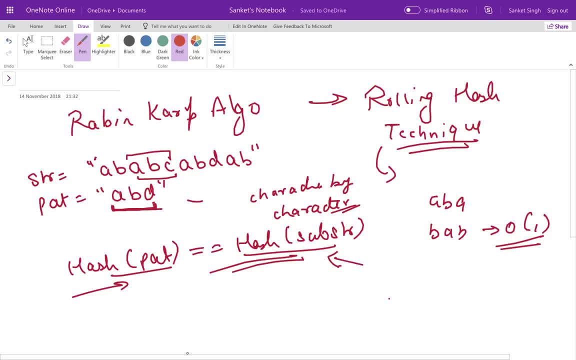 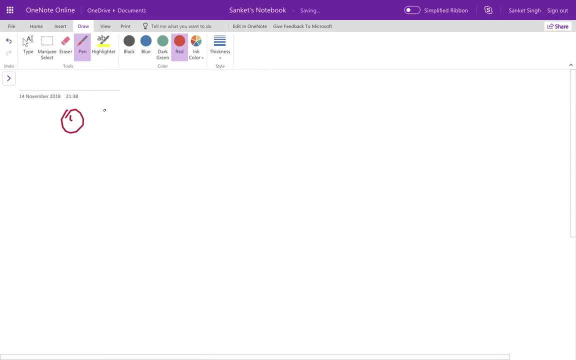 will see that if all the characters match, If all the characters of the pattern matches all the character of the substring, then we have found a match. else we are not finding any match and we will continue our algorithm. So what we will do in Rabin-Karp algorithm is initially calculate the hashes of the new 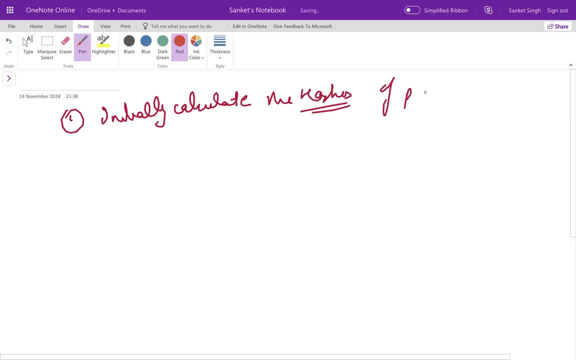 substring of pattern and the first substring. and then what we will do is that once we have got the initial hash values of our pattern and the first substring, we will try to iterate over the whole given substring in a particular window size And then we will check if the hash value of the new substring matches the hash value of. 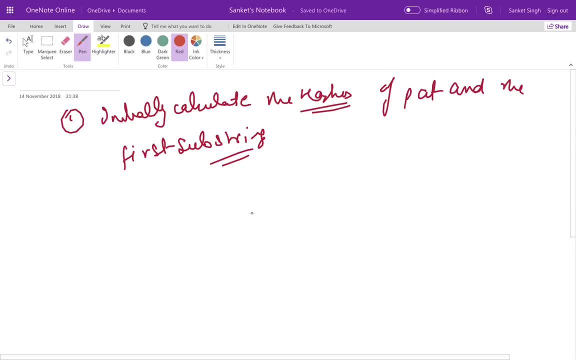 the pattern or not And if our current hash value matches the hash value of the pattern or not. And if it matches, then we will double check by iterating over the pattern and substring to check if all the characters of the pattern are matching, all the characters of the given. 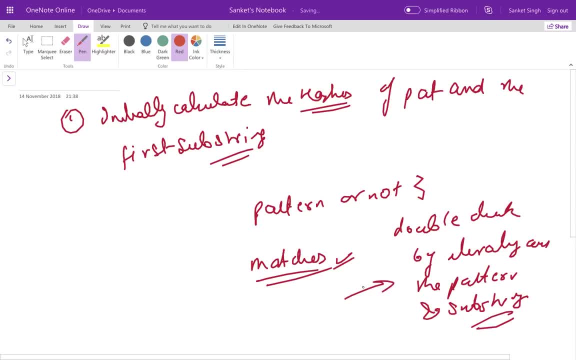 substring or not. Why we are applying this double check is because, suppose, if we have not implemented a very good hash function, then there is a possibility that for many substrings of the given string the hash value matches the hash value of the pattern. So the bad- our hash function is the bad- how code will run. 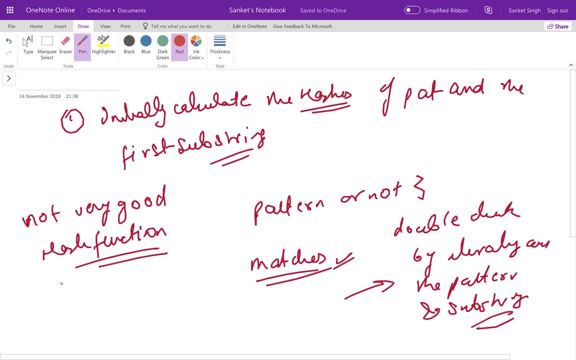 So we will try to implement as efficient algorithm as possible, because if Rabin-Karp algorithm performs poorly and every next substring has a hash value that matches the hash value of the pattern, Then our code will run in troll по and sen н пожалуйста. 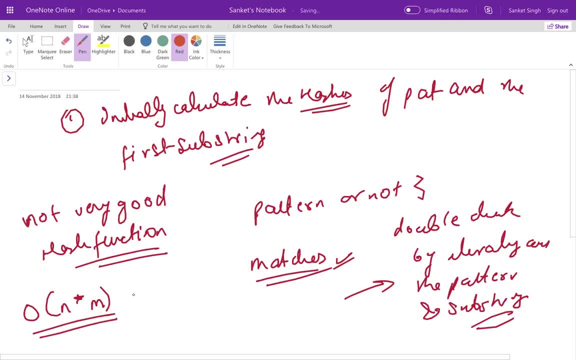 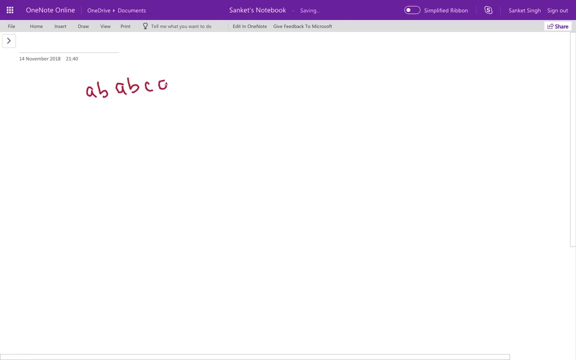 O of n into m time, complexity only. That is very similar to our brute force approach. So what I am trying to say here is that suppose let us take an example. So for the given string a b, a, b, c, a b, d, a b and the given pattern a b d, So 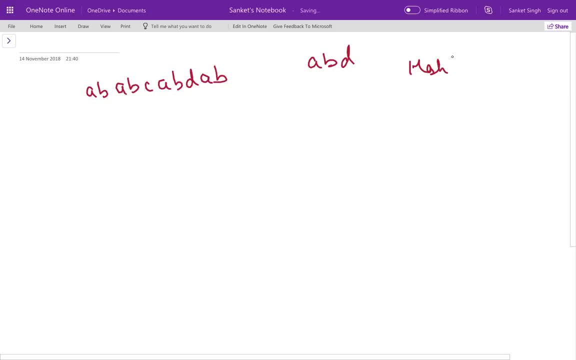 let us suppose that we have a hash function and it takes a, b, d and gives 33 as the hash value, and we will start the window with a, b, a and calculate the hash of a, b, a and it gives the hash as 54. So here you can see, the hash values are not equal. So what we will do is shift this. 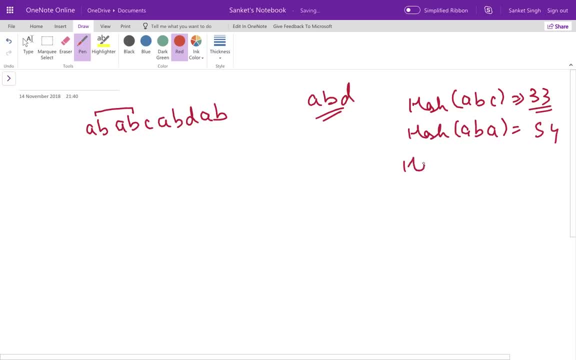 window to the next eligible substring, b a b. So we will calculate the hash of b a b and suppose the hash value of b a b comes out to be 19.. So here you can see the hash values are not equal. So there is no chance that. 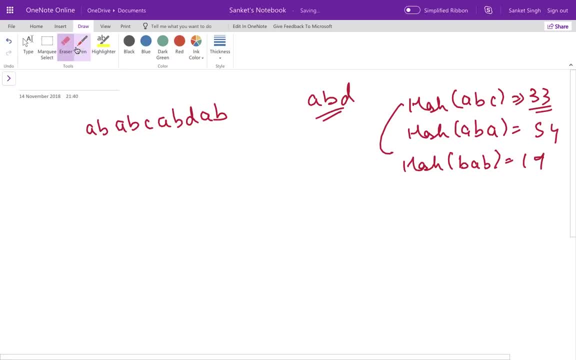 the substrings will be equal. So here we will again shift this window to the next eligible substring. So the hash of a b c will be calculated, and suppose this hash comes out to be 33.. But as you can see, a b c is not equal to a b d. 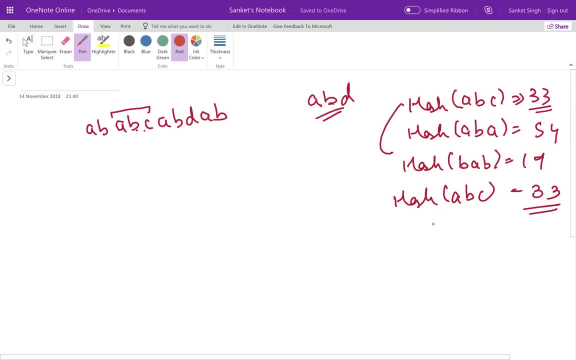 So it is very important to check that if the hash values matches, then also the characters are matching to our particular substring. So by matching each character by character, we will see that here at the last character we have found that the characters are not. 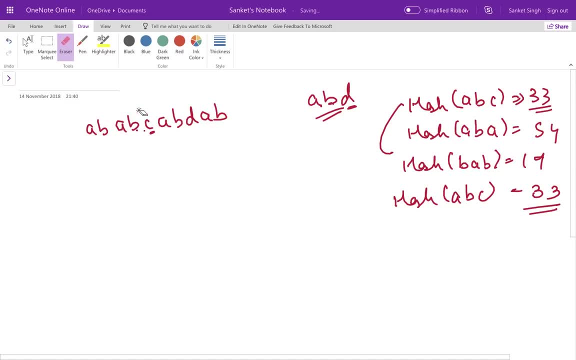 matching and then we will again shift our window to the next eligible substring. So that is b c a. Suppose the hash value of b c a also comes out to be 33.. So here you can see the hash function is working very poorly and for substrings. 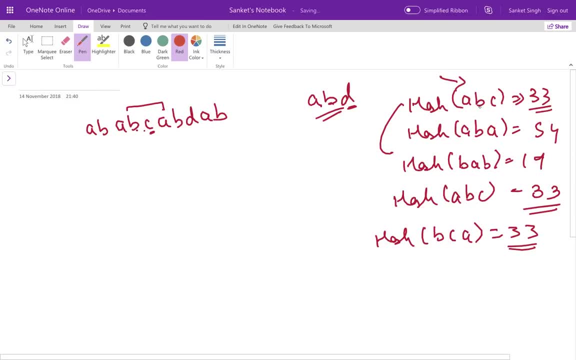 that are not equal to the initial substring, or I can say I should say the substring of the pattern. it should be a, b, d, So the substring that are not equal to the pattern is all- are also giving the similar hash values. The hash function is not working as as properly as 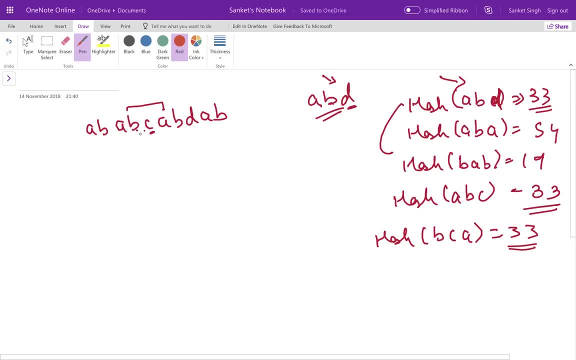 expected. So here we also have to double check if the characters are matching or not. and here you can see the characters will not match and we will shift our window to the next eligible substring, c a b. So the hash value of c a b will be calculated and suppose 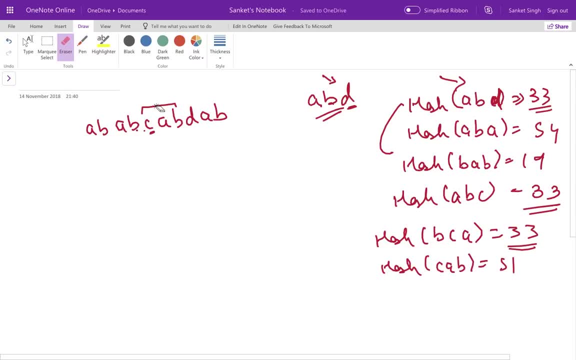 the hash comes out to be 51. Then the hash value of a, b, d will be calculated. So the hash value of a b d will be calculated and this will definitely come out as 33, because initially our hash function gave 33 for a b d. So here also we have to double check. 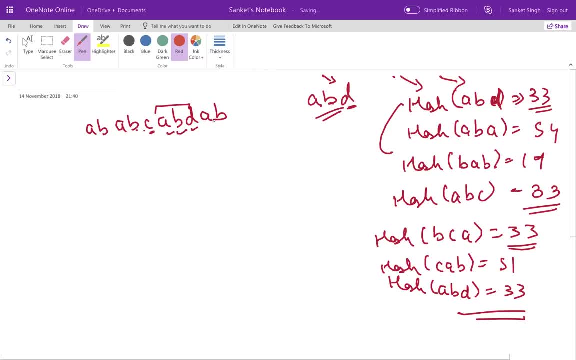 if all the characters are matching or not, and here you can see all the character of the given substring will match the given pattern. So we will return the index of this a. So if our hash function will work efficiently, then at max what we will be doing is iterating. 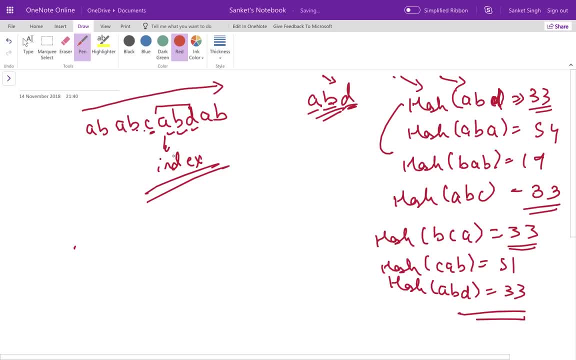 over this whole string and if there is any match in the hash values, we will be checking the given pattern for the characters. so the, so the average case time complexity will come out to be O, which is very fast than brute force. so here you can see we have optimized. 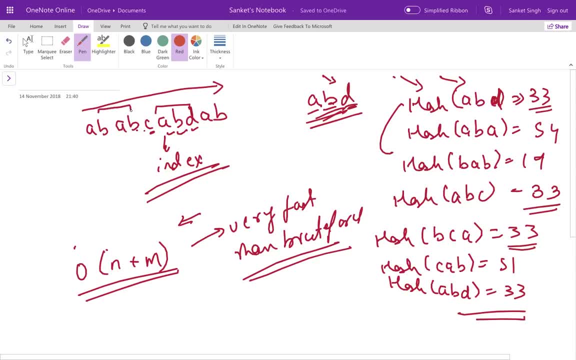 our solution, as shifting the window and calculating the new hash is taking constant time, that is, we go off one time. so we have optimized our solution using the rolling hash technique. so here you can see that if we were using the brute force we were getting the time complexity. 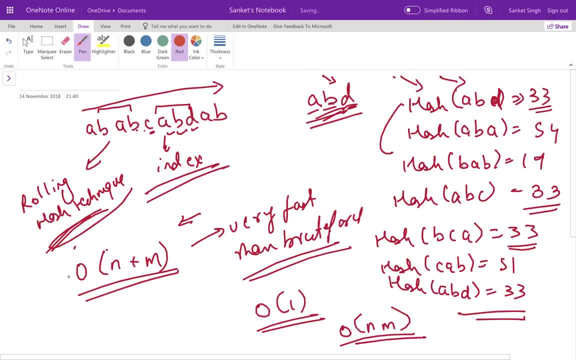 as n into m, and here the average case time complexity will come out to be a little bit less, but still the worst case complexity for Rabin-Karp can be as bad as we go off n into m. and when will this situation occur? this situation will occur if our hash function. 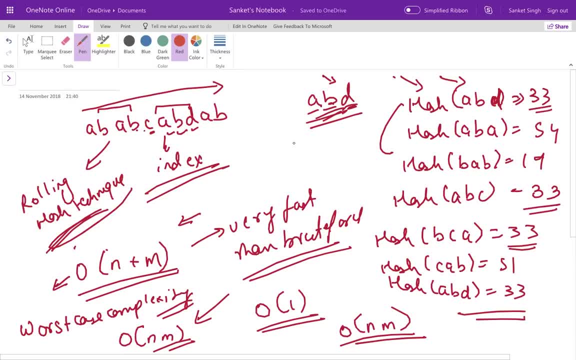 will repetitively give similar hash values for different substrings. so I hope the logic is clear to you all. What are we all have to do is initially calculate the pattern hash and the hash of the initial substring of length equal to the pattern length, and then iterate over the whole string and one. 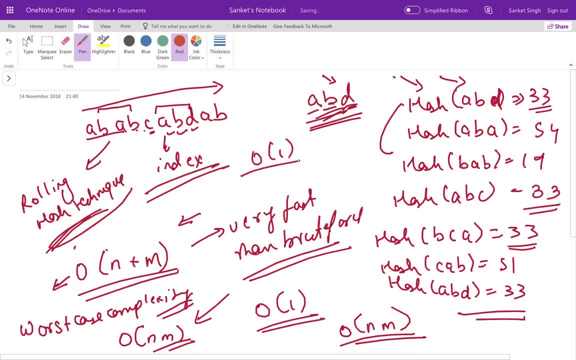 by one calculate the new hash values in big O of one time complexity using rolling hash, and then if anywhere the hash value matches, then we have to manually check the whole substring, that if the substring matches completely with the given pattern or not. and if it matches then we will return the index, and if it doesn't, does not match, then 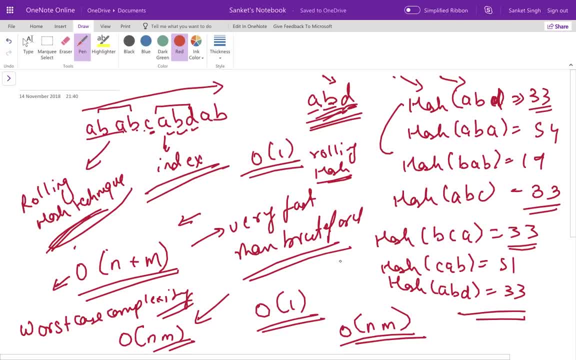 we will iterate over the next eligible substring. so I hope you all have got a clear perspective of how Rabin-Karp algorithm works. try to implement this algorithm on your own and then in the next video we will try to implement this algorithm. thank you.